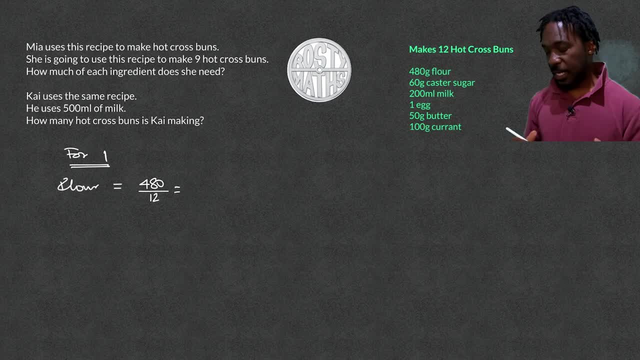 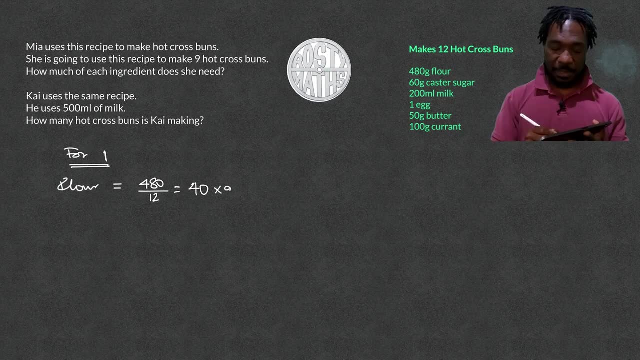 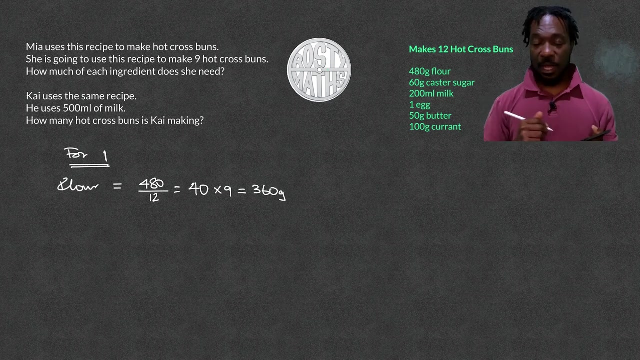 going to say 480 grams of flour divided by 12. That is going to give me 40 grams. Now all I need to do is multiply that by 9 to then work out that I need 360 grams of flour. I'll do it again. I'll. do it again. Let's look at the sugar. So you got the caster sugar there Again. find out how much to make one. So to make one, I need 60 grams of sugar divided by 12. That's going to give me 5 grams of sugar to make. what one hot. 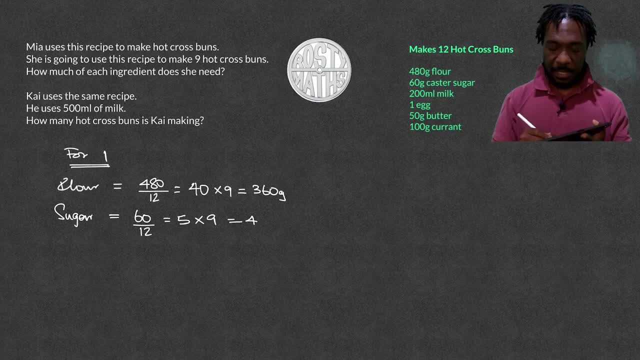 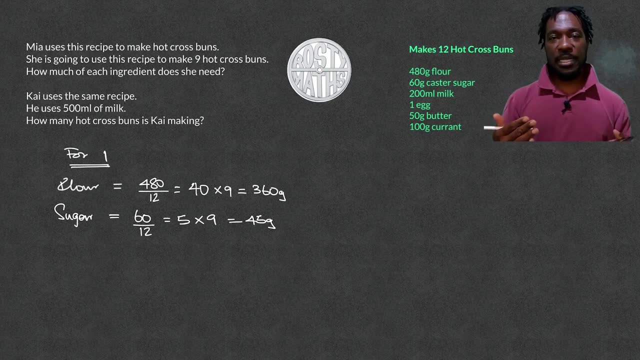 cross bun. I times that by 9 to work out that I need 45 grams of sugar. All right, cool. What I'm going to do is I'm going to pause the video here. Do the rest of them, and then we will talk about. 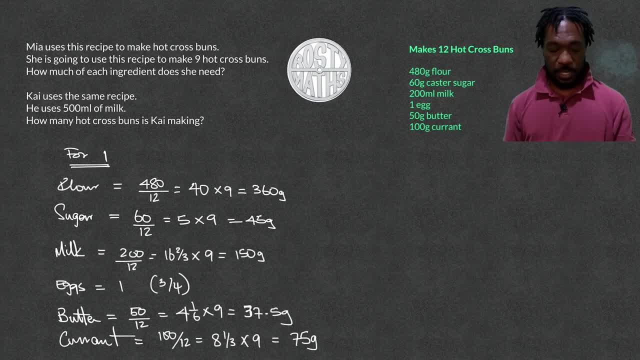 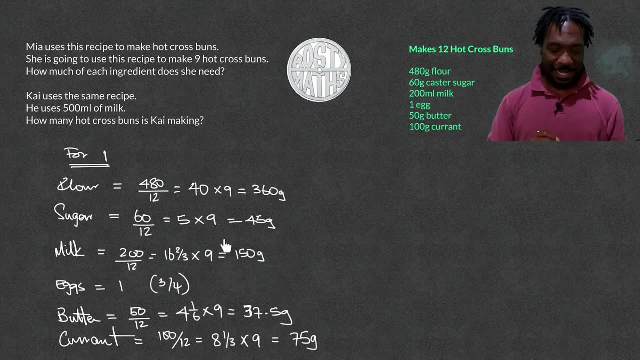 that second method. So here is all the working out. Now there's something I want to point out here is that when I was making 12 hot cross buns, you needed one egg. Now, when I tried to make for 9, it tells me I need three quarters of an egg. If you want to go try and measure out three quarters of 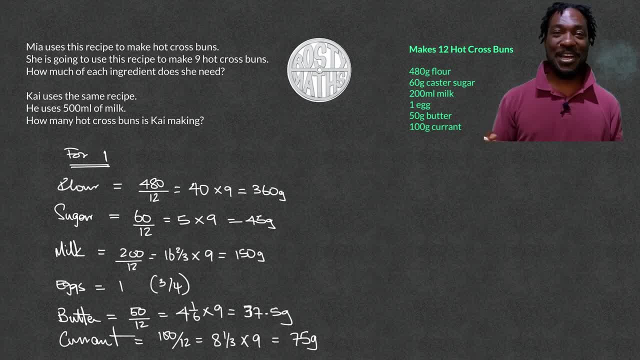 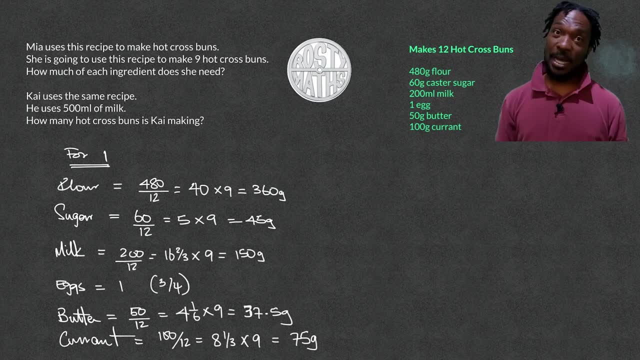 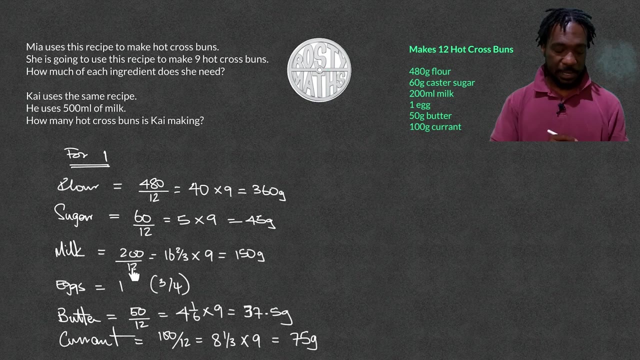 an egg. be my guest. I'm pretty sure in the comments below somebody who does their recipe will tell me: yes, you need three quarters of an egg, Mr Ross. Okay, I'll just put an egg in just to be on the safe side, But anyway, that's beside the point. As you can see, I've followed the same method: Divide. 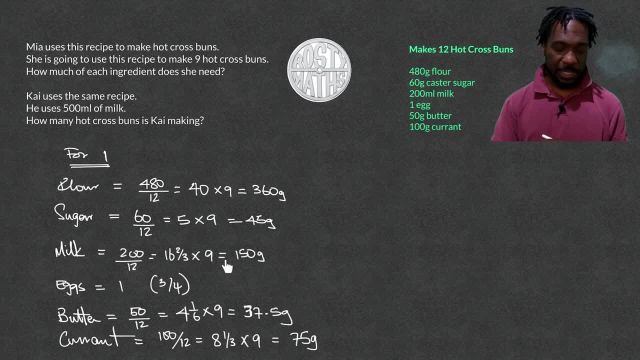 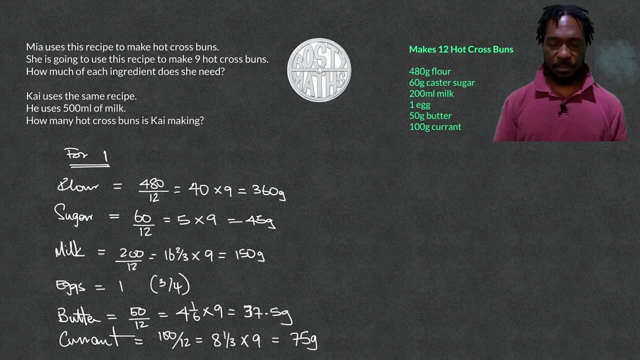 the number that I've got there: 12 to work out for 1, and then times by 9.. So these are my different ingredients here. Now let's talk about that all important second method. Now for the second method. what I'm going to do is I'm going 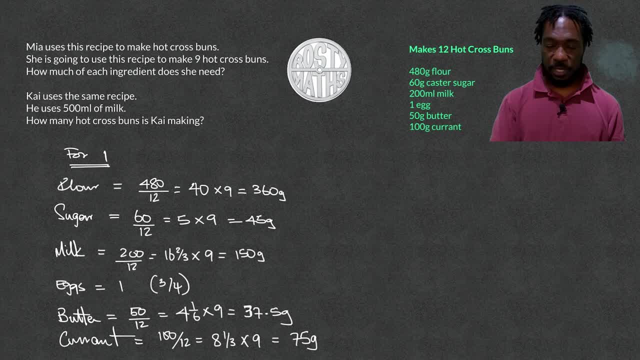 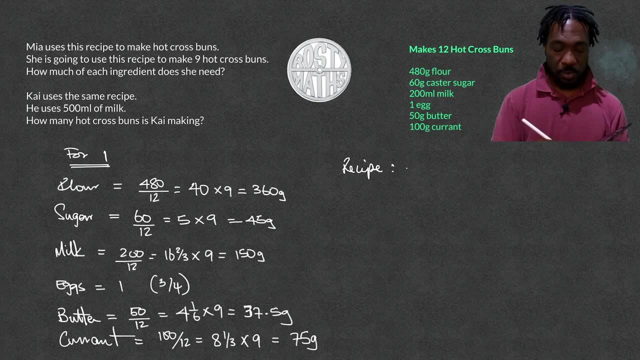 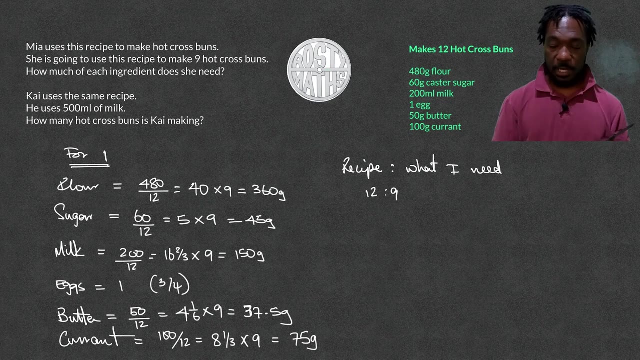 to represent my different servings as a ratio. So, for example, the recipe- to what I need. I'm going to say what I need is 12 to 9. Because the recipe makes for 12. But I only need 9.. So how do I use this now to work out how much of 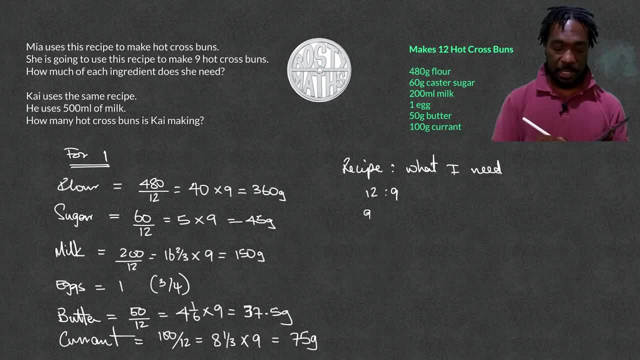 each ingredient I need, Simple. I only need 9 twelfths of that whole recipe because I don't need a full 12.. So I just need to do 9 twelfths and I multiply that by that 480 for my flour and I will. 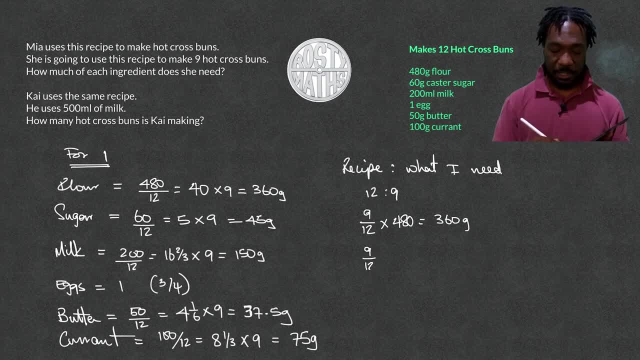 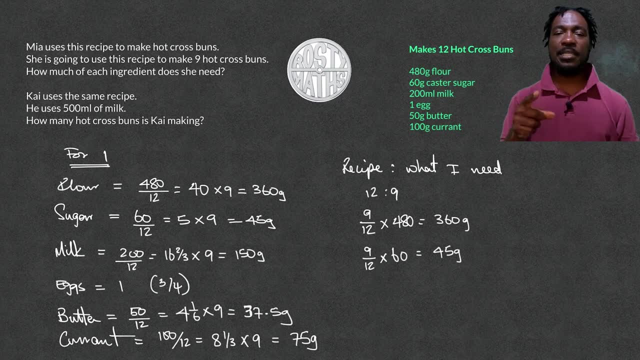 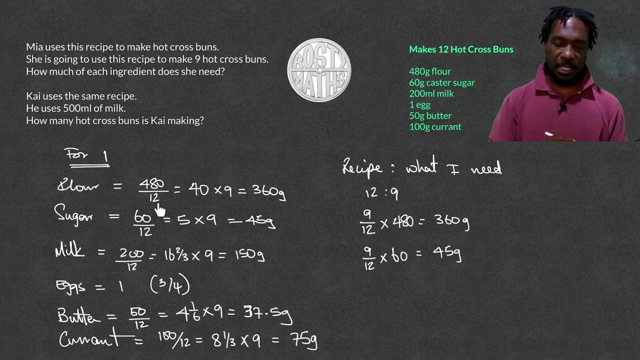 still get 360 grams. I do my 9 twelfths and I multiply that by 60 and I will still get 45 grams. Now, why did I say that? it's the same method done in two different ways? Well, here's why I said that In this method, when we were 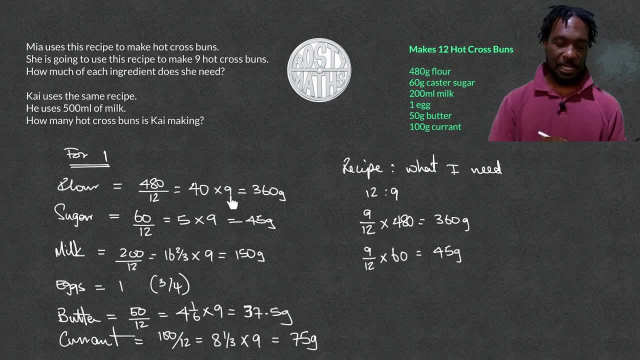 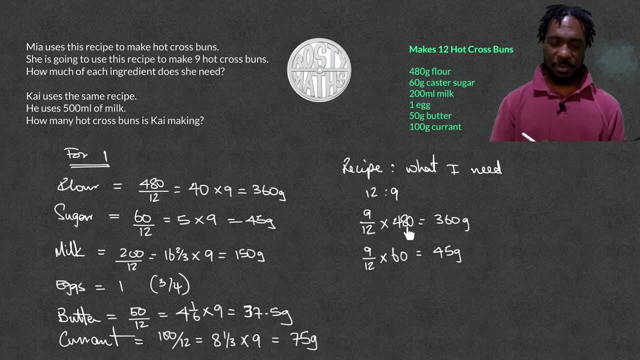 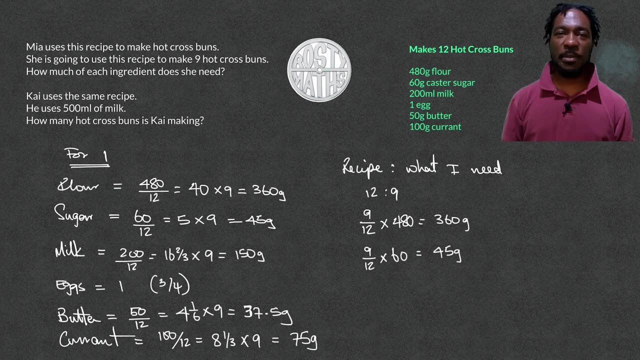 finding: for 1, we divided by 12 first, and then we multiplied by 9.. How do we work fractions out? Similar thing, isn't it? You divide by 12 first, and then you multiply by 9, and you get that. Which method worked for you? Drop it in the comments below. Now, let's do that last part of. 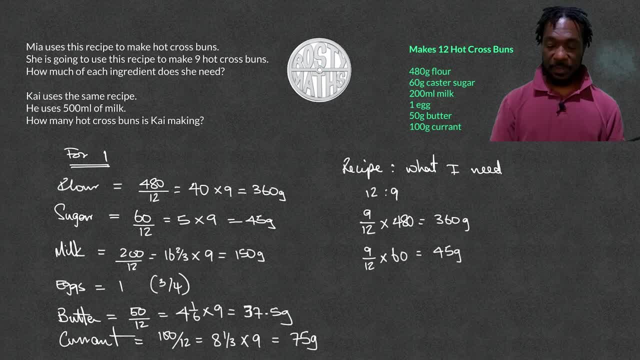 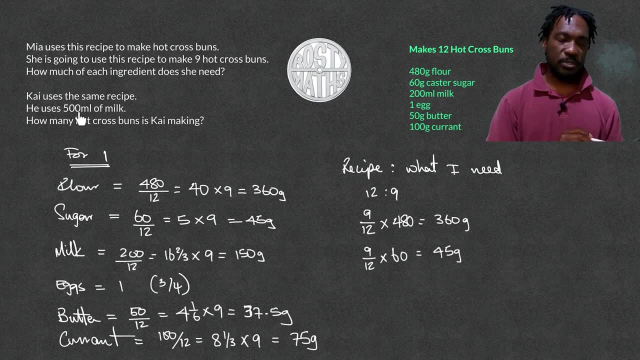 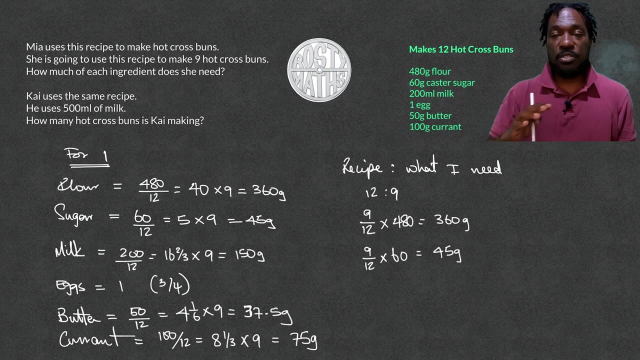 the question and finish up this video for today. Now, the last part of the question says Kai uses the same recipe, This same recipe, here. He has 500 mils of milk. How many hot cross buns is he making? So we're going to assume that he's going to use all of the milk that he has Now, if he's only got 500 mils? 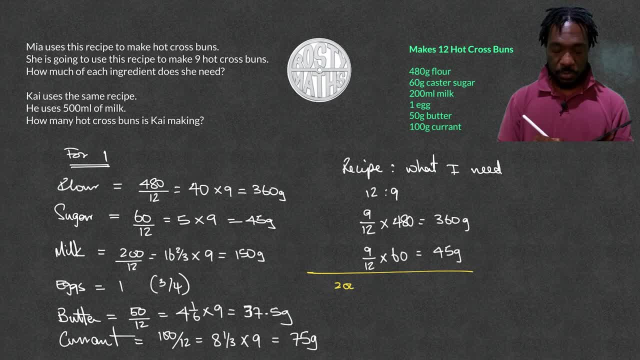 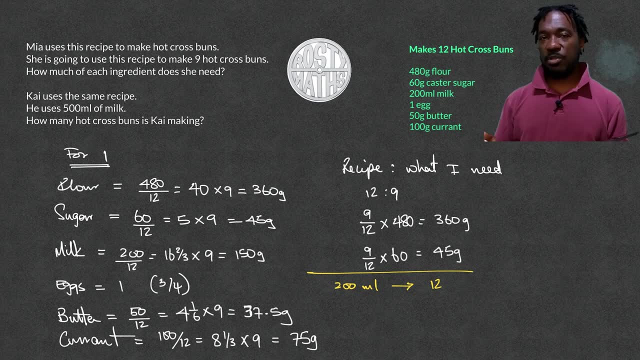 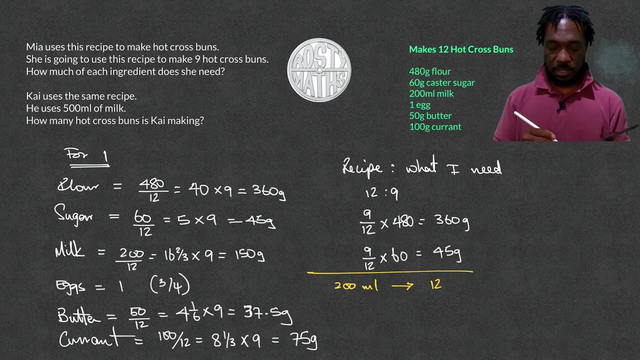 Let's remind ourselves of a few things. okay, 200 mils of milk makes 12 hot cross buns. But now he's got 500 mils of milk. How do I work out how many hot cross buns he's going to make? Well, simple job. All I've got to do is take that 500 mils of milk. 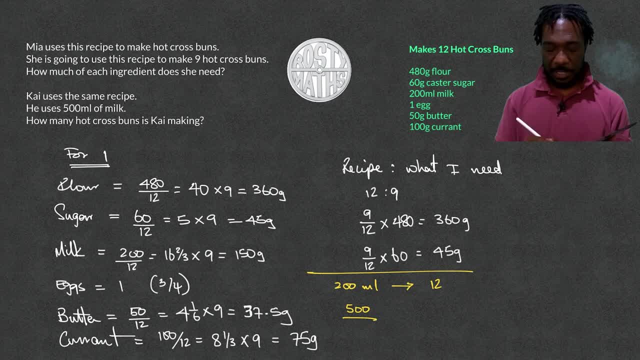 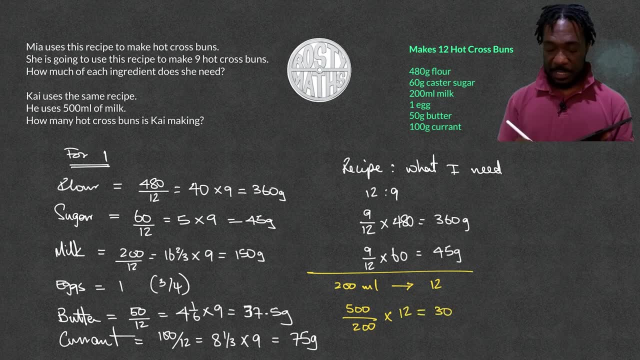 Divide that by the 200.. Let's make sure we write 200 mils of milk there and multiply that by 2.. 12, and then this is going to give us that he's making 30 buns. Now you might want to know why did. 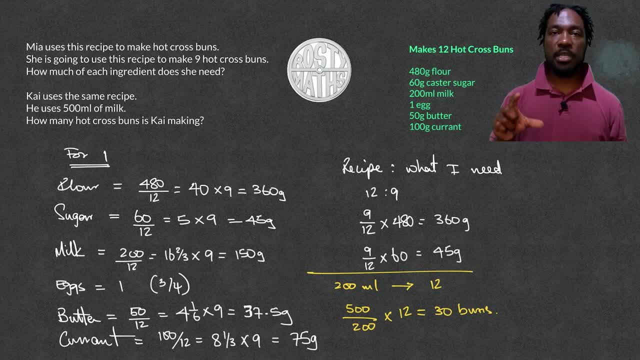 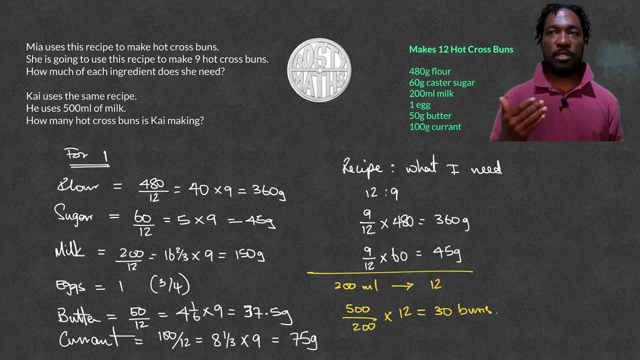 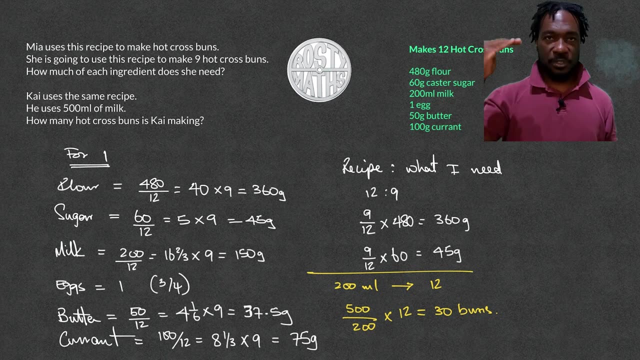 I do that. Okay, the reason why I do that is because I want to find again the proportion of the original amount that he's making. So he was making he had 200 mils of milk and now he's got 500. So the proportion that he's got is 500 divided by 200. When I have that proportion, I just